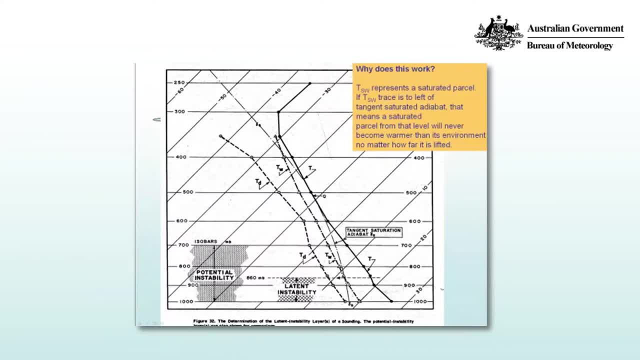 point temperature profile, the dashed line. If you lift parcels to saturation from every pressure and bring them back down to the original pressure, you get the wet bulb temperature. And so, calculating the wet bulb temperature at every pressure level, we can build up the 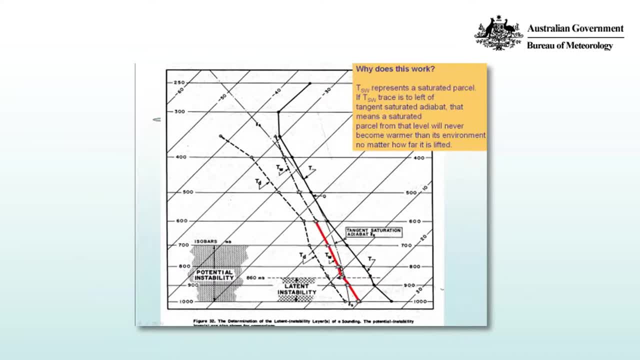 wet bulb temperature profile like so at each and every pressure. Then we mark in the tangent saturation adibat And you can see it's the saturation adibat with the lowest temperature that just grazes the temperature trace here at point Q. Now consider parcels of air on the wet bulb temperature profile to the left of the saturation. 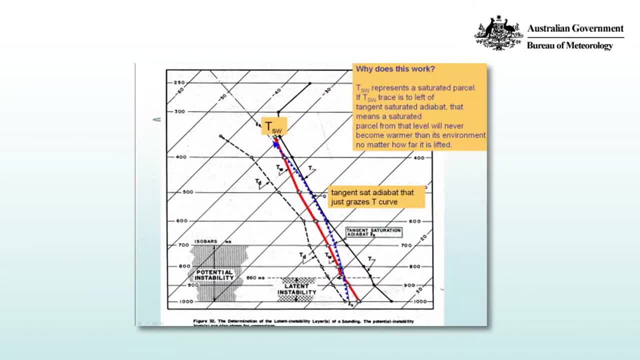 the tangent saturation adibat. Parcels lifted from this curve will follow a saturated adibat And the saturated adibat along which they ascend will never cross the temperature profile, Whereas parcels of air lifted from the wet bulb profile to the right of the tangent saturation. 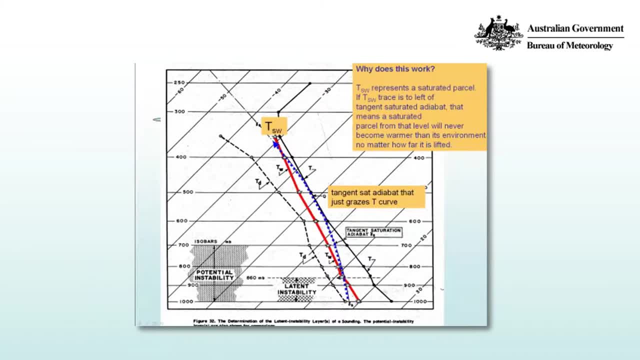 adibat will ascend along. saturated adibats that eventually cross the temperature profile, become warmer than the environment and therefore are unstable. So in this case, below 860 hPa parcels of air are said to be latently unstable because eventually they will cross the temperature profile and become unstable. 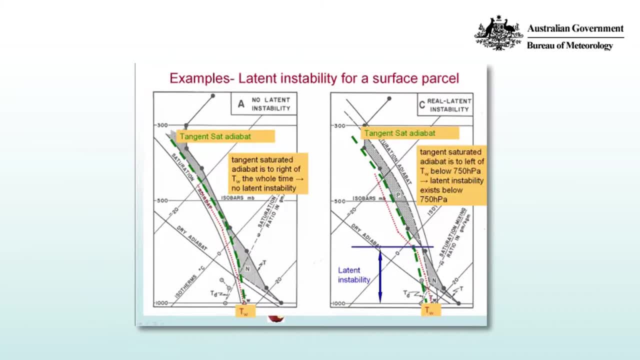 In this figure. here we see an example on the left where a surface parcel has no latent instability. The tangent saturation adibat is marked in green and the wet bulb temperature for the surface pressure will move along a saturated adibat represented by the red dotted line. 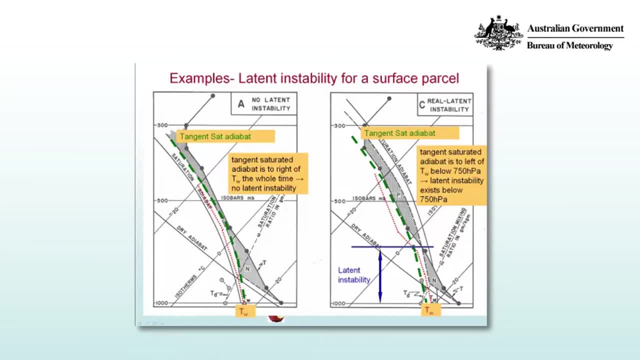 This line is to the left of the tangent saturation adibat and indeed to the left of the temperature profile, and therefore no amount of lifting will release instability. Compare that to the figure on the right, where the tangent saturation adibat again is marked in green. 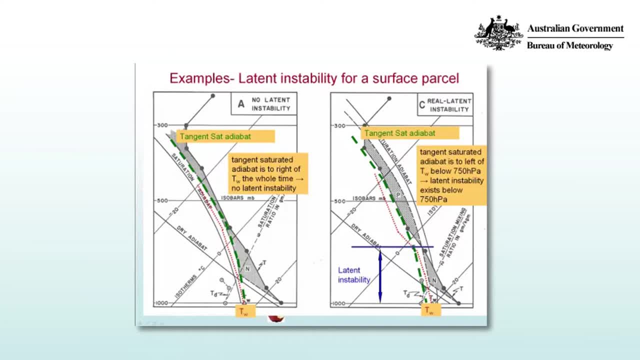 and we've got a wet bulb profile marked in red. The surface parcel possesses latent instability because as it lifts along a saturated adibat, it eventually crosses the profile. In fact, we can see that below 750 hPa the atmosphere contains latent instability because 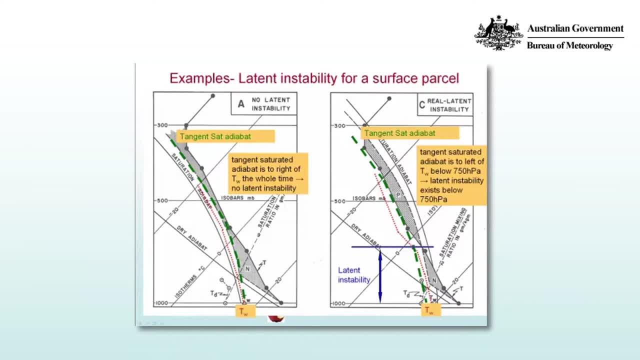 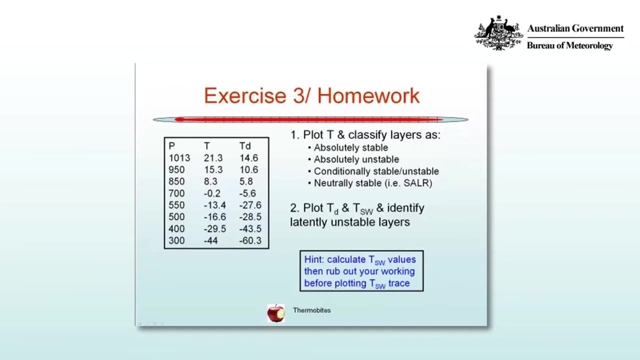 all parcels of air below 860 hPa are not unstable. In fact, below 750 hPa, the wet bulb temperature lies to the right of the tangent saturation adibat. Exercise 3. Plot the temperature profile and classify the layers according to their static stability. 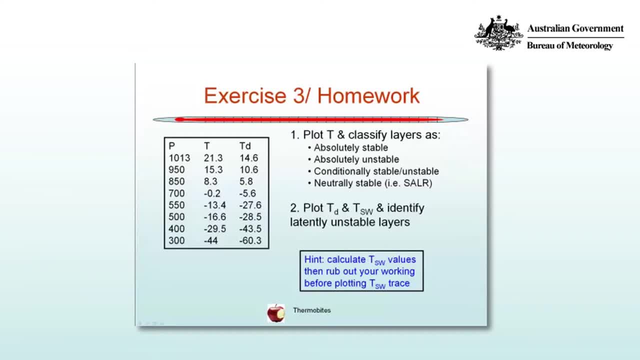 Then plot the dew point profile and the wet bulb temperature profile and identify layers as unstable in a latent sense. As a hint, when you calculate TSW, once you've marked in the dry adibat and the mixing ratio line up which the parcels moved and the saturation adibat along which the parcels moved back down. 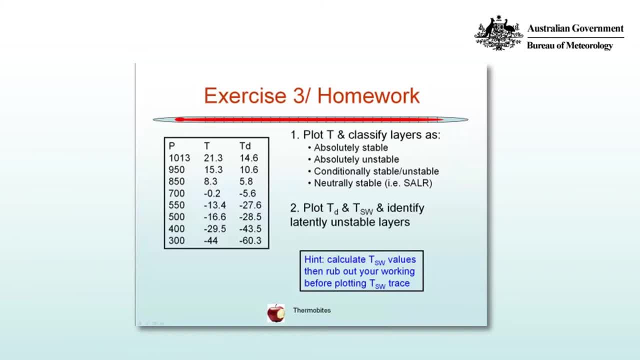 to the original pressure. you want to rub them out. So pause the video now and complete this exercise, either as an exercise now or as homework. So how did you go? Here we have the lower parts of the profile And then we have the adibat in the lower part of the profile and the dry part in the lower part of the profile. 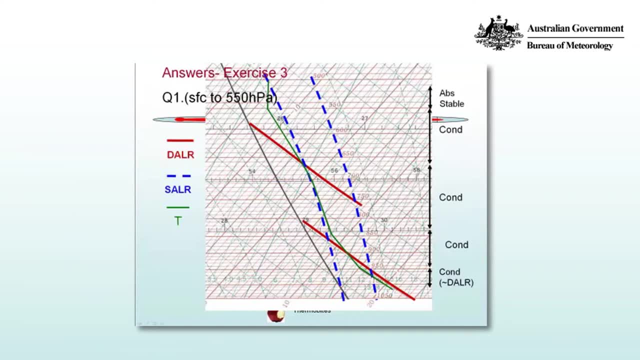 So this is my exercise now and the green line is the temperature profile and the red line here is a dry adiabat and the blue dashed lines represent saturated adiabats. You can see in the lowest layer. it contains conditional stability or instability. 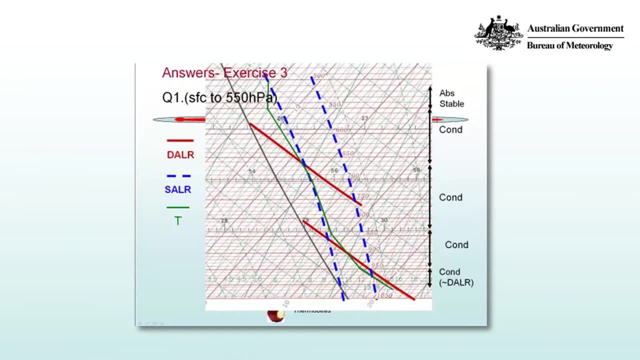 because it's approximately a dry adiabatic lapse rate. Parcels must be saturated Again. for the second layer and the third layer there's conditional instability, and indeed the fourth layer. It's not until we get to the fifth layer that we see that it's absolutely stable. 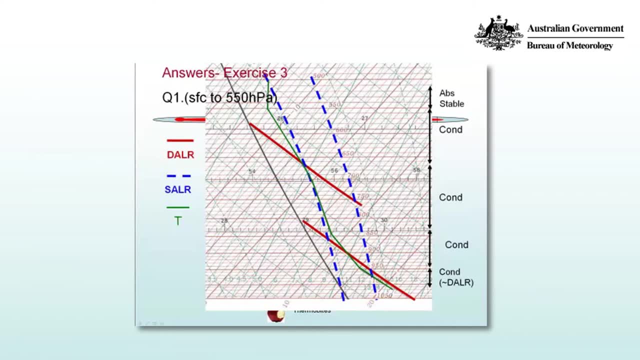 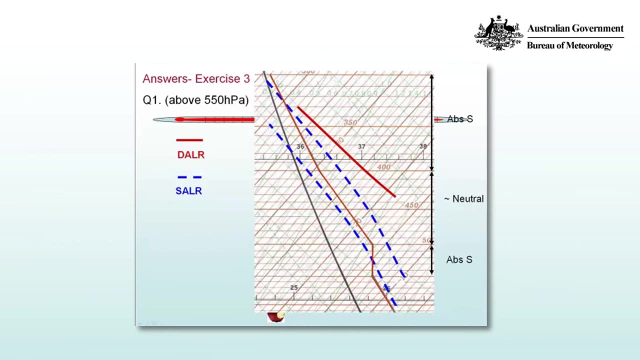 because parcels of air moving along that blue saturated adiabat become cooler than the environment. For the upper part of the atmosphere we see an absolutely stable layer and then an approximately neutrally stable layer where the temperature lapse rate is about that of a saturated adiabat. 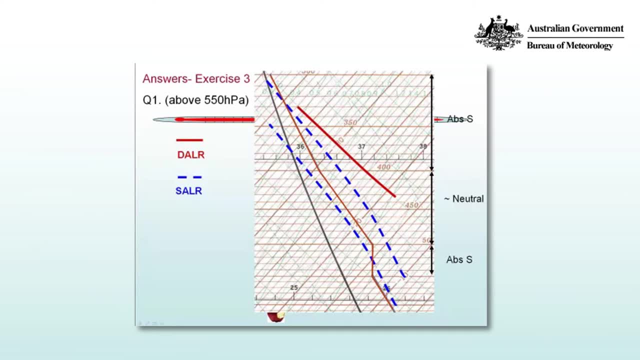 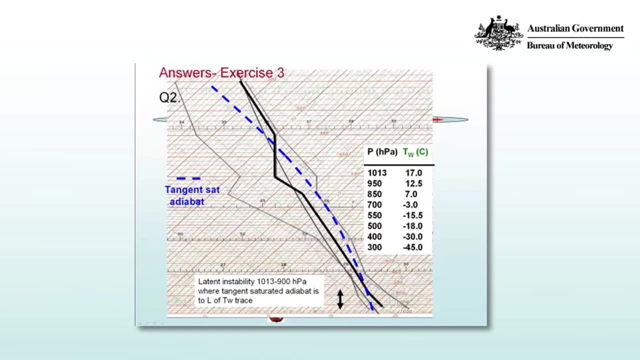 Finally, the top of the atmosphere here is absolutely stable. Here are the values plotted. Here's the value of the wet bulb temperature and you'll note there's an error in the plotting of the wet bulb temperature at 500 heteropascals. 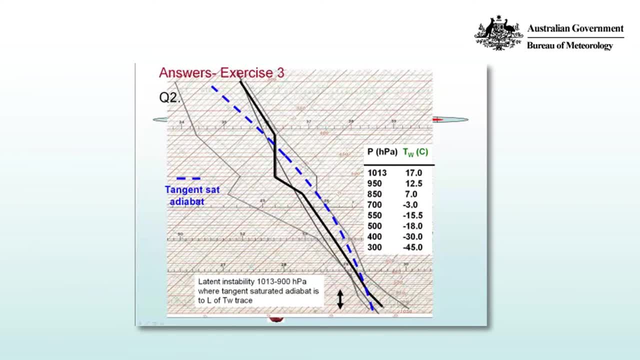 The value in the table is correct, You can see that the tangent saturated adiabat touches the profile and actually grazes it in the region of atmosphere that approximates the saturated adiabat, so it doesn't just touch at one point.